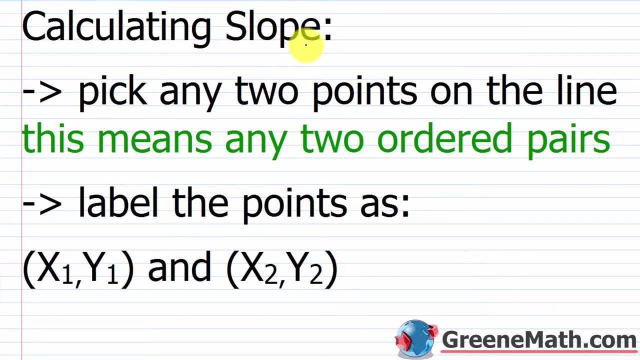 a little while So calculating slope, and this is using the slope formula. You're going to pick any two points on the line and you're going to use the slope formula, And then you're going to use the line. It doesn't matter which two points you pick. So this means any two ordered pairs And 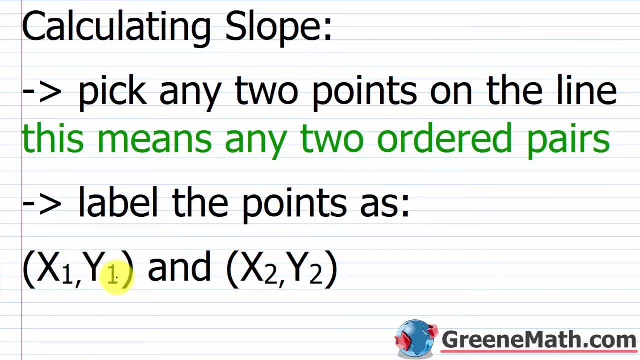 you're going to label the points as x sub 1, y sub 1, and x sub 2, y sub 2.. Now let me stop. I'm introducing some new notation, so I want to clarify This right here. this one, that's kind. 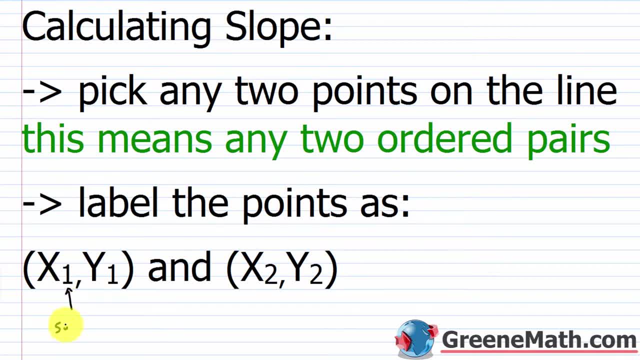 of sitting next to the x is read as sub 1.. This two, that's sitting next to the x, is read as sub 2.. This is a way for us to notate that we have two different x values that we're thinking about here. 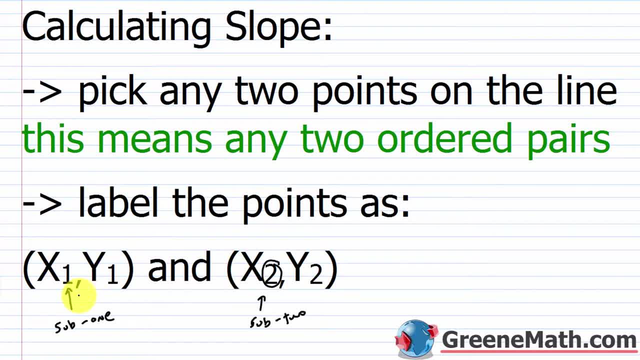 without actually kind of changing variables. right, And in a lot of math I can just pick a variable, a different letter every time I have something else I'm representing, But here, because we're specifically thinking about, okay, the x value is the value that we're thinking. 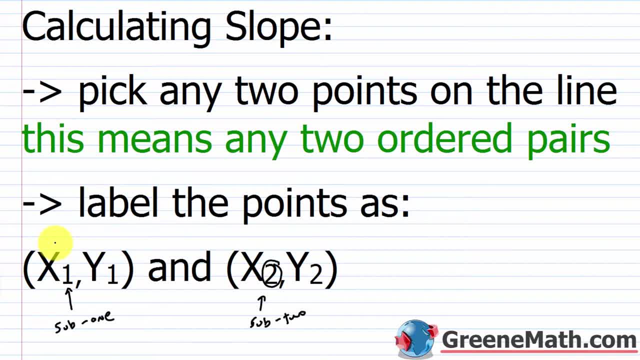 about. that corresponds to the horizontal axis. So I've got to be consistent there. I can't say, okay, I have x and then I have some variable named z. That wouldn't make any sense. So we have to have two different x values, And so to separate them we use sub 1 and sub 2.. If I was working, 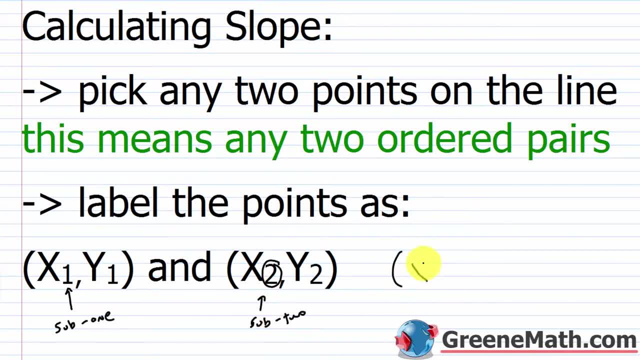 with something that had three different x values, I would have a point that would be x sub 3, y sub 3, right, So on and so forth, And you're going to see that as you move higher in math. when it calls: 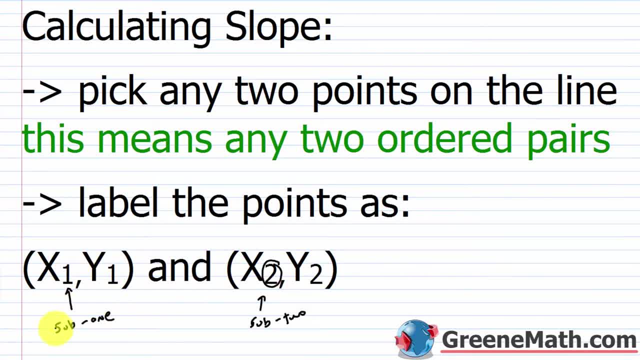 for that, But for right now we just need two. So that's where this is coming from. So you have x sub 1, y sub 1, and x sub 2, y sub 2.. Now the next source of major confusion is: which point do I? 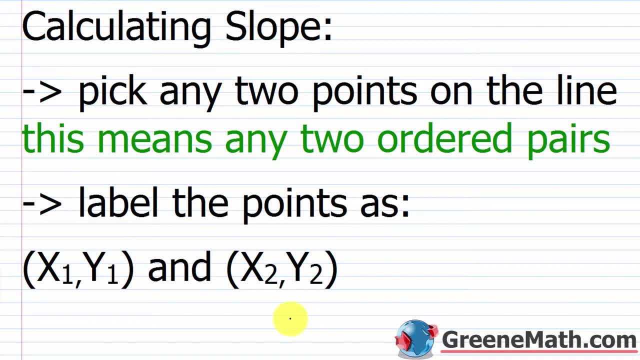 label x sub 1, y sub 1?? And which point do I label x sub 2, y sub 2?? And the answer is: it does not matter. Okay, and I'm going to show you that so that you understand, because I can't tell you how. 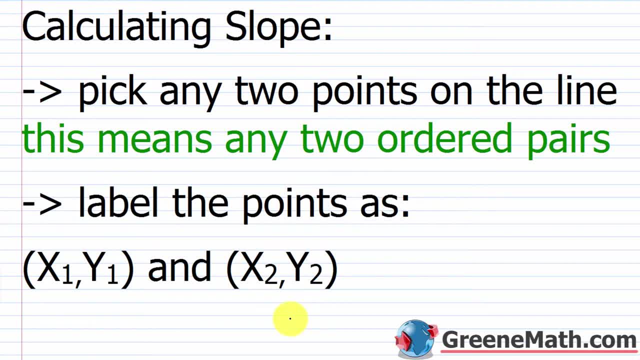 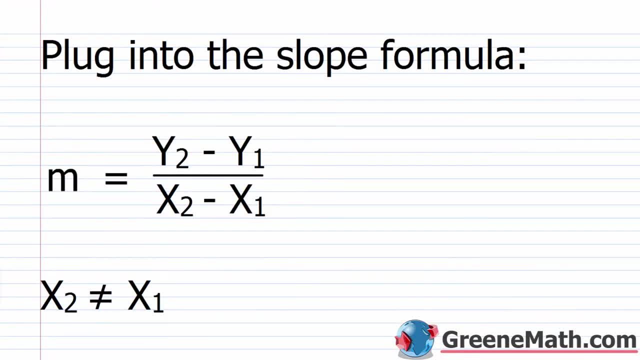 many people come up to me and say: well, how do I know which one to label is, which It does not matter, You can switch them around, you're going to get the same exact answer. So once you've labeled them, all you need to do is plug it into the slope formula. 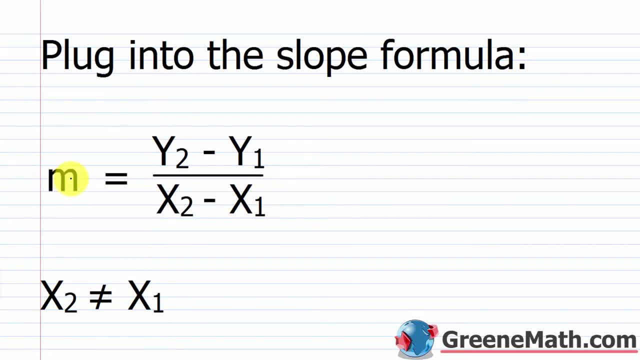 And I advise you to copy this down. We have that m which stands for slope, This stands for slope, And I don't know why m stands for slope, but it does, And this is equal to. we have y sub 2 minus. 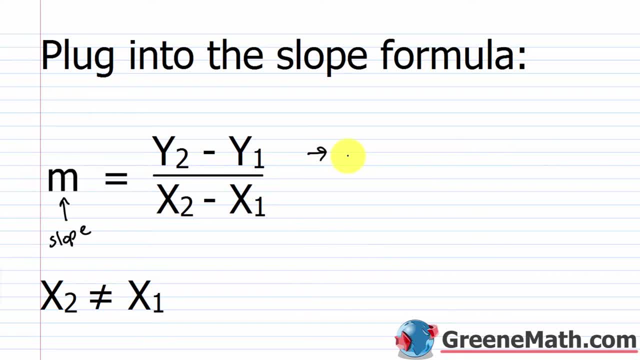 y sub 1.. So this is referred to as your change, your change in y values. And then this is over. we can think about it as dividing by x sub 2 minus x sub 1, which is what It's: the change in x values. Okay, the change in x values. So we have the change in y values over. 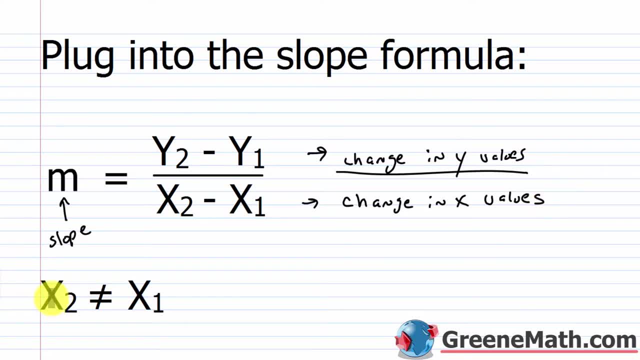 the change in x values. And then one important note: we can never have the case where x sub 2 equals x sub 1.. Why? Because we can't divide by zero. If I have the same number here, let's say 2 and 2,, 2 minus 2 is 0, I can't divide by 0. So that's a problem. So x sub 2 cannot equal. 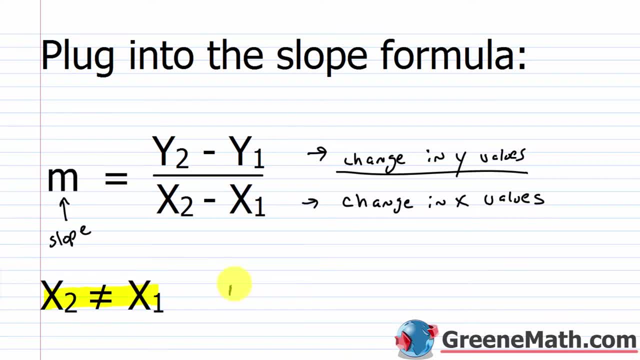 x sub 1.. And another way we might see this written is that m our slope is equal to the rise over the run, And this is just a way to remember that it's the change in y values or the rise. you can think about this as going up and down over the change in x values or the run. You can 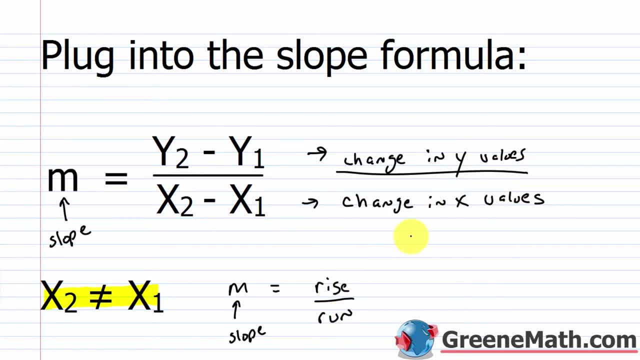 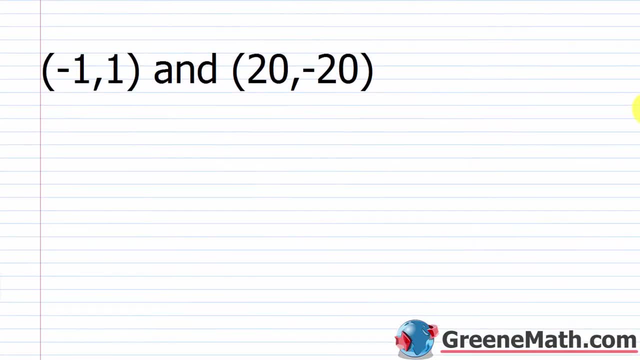 think about running as going up and down, And this is just a way to remember that- it's the change in x values or the rise over the run. So we can never have the case where x sub 2 equals x sub 1.. Okay, so let's start out with two points. This is a typical example of something you see on your 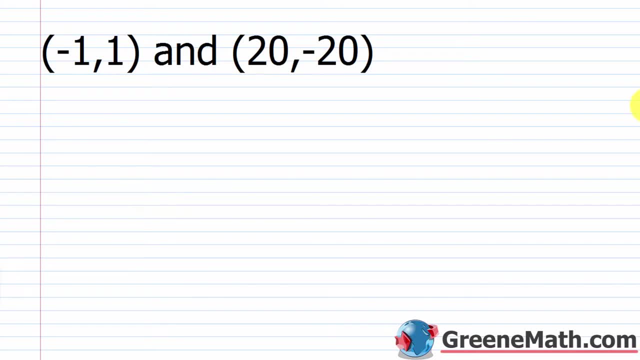 homework or tests. You're given two points and you're asked to calculate the slope. So we have the point negative 1 comma 1 and 20 comma negative 20.. So the slope formula is: m equals y sub 2 minus y sub 1 over x sub 2 minus x sub 1.. And I'm not going to write this out, I'm just going to. 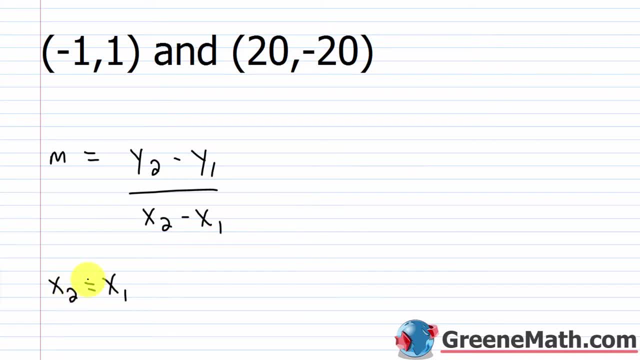 every time. but remember that x sub 2 is not allowed to equal x sub 1.. It cannot. All we need to do is label one of these points as x sub 1, y sub 1, and the other x sub 2, y sub 2, and then. 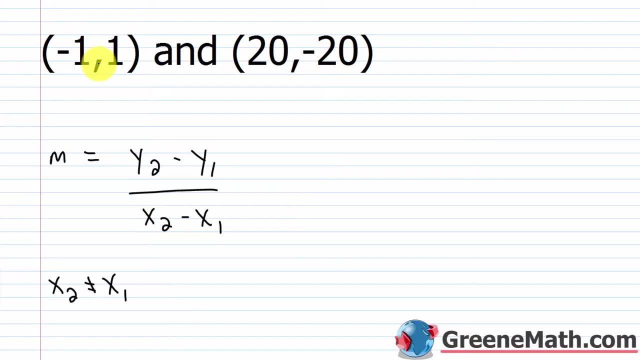 just plug in Again. it does not matter which point you choose to be x sub 1, y sub 1, and which point you choose to be x sub 2, y sub 2.. It's completely irrelevant. You get the same answer. 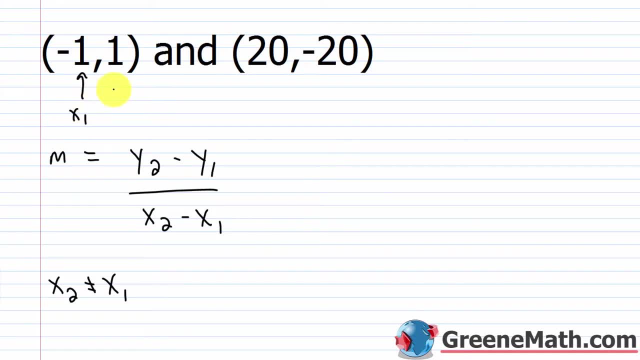 either way. So I'm going to pick this to be x sub 1, y sub 1, and I'm going to pick this to be x sub 2, y sub 2.. One thing that you cannot do, okay, you cannot mess this up in terms of saying: 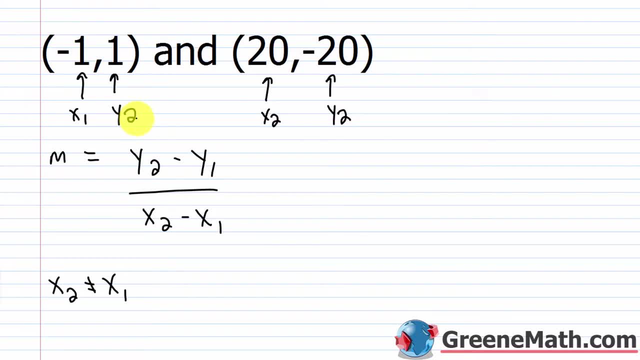 well, this is x sub 1, y sub 2, and this is x sub 2, y sub 1.. That will give you the wrong answer. Do not do that. If this is x sub 1,, this has to be y sub 1.. If this is x sub 2,, this has to be: 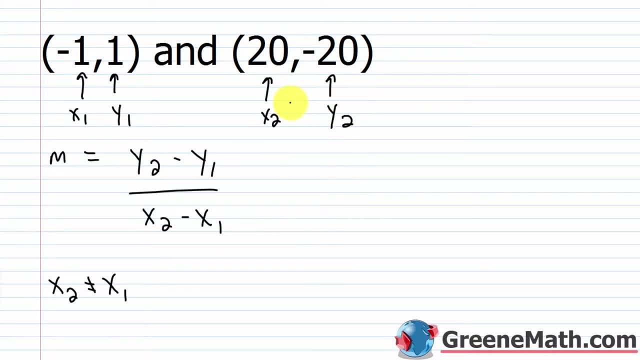 y sub 1.. y sub 2.. Now, you cannot mix those numbers up like that. Now, once you have labeled everything, go ahead and just plug into the slope formula. It's really just that simple. So I have y sub 2 here, So I'm going to take negative 20 and plug that in. So let me just 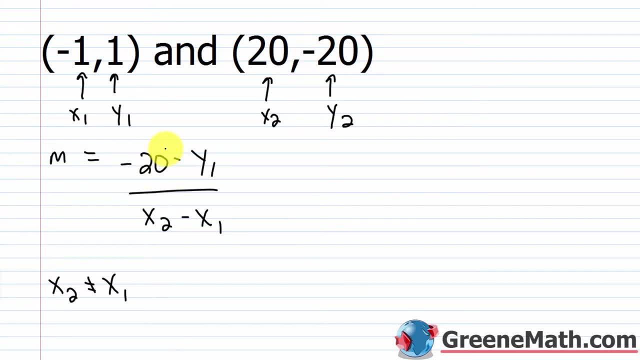 erase this and just put a negative 20 here in its place, And then I have minus. I have y sub 1.. So that's 1.. Let's erase this and put 1.. And then I have x sub 2 down here, That's 20.. So erase this. 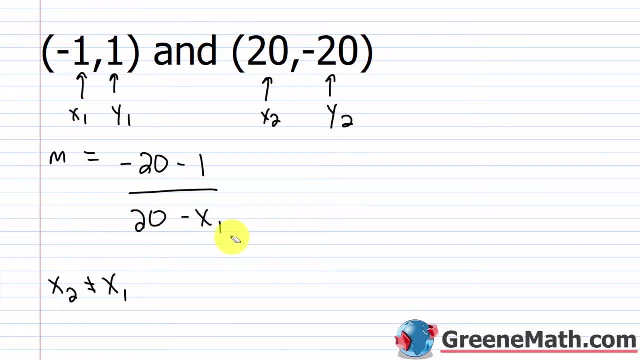 and put 20.. And then for x sub 1, I have negative 1.. So let's erase this and put a negative 1.. Now, again, again, again. it's very important to pay attention to your signs when you're. 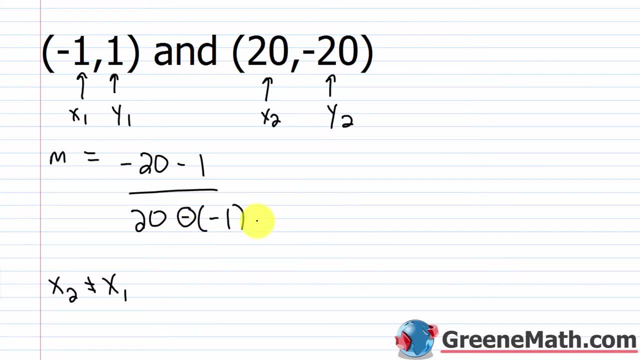 plugging in for something. I already had a negative out in front. I'm plugging in a negative 1 for x sub 1. So it's minus a negative 1.. Don't make the mistake. Don't make the mistake. 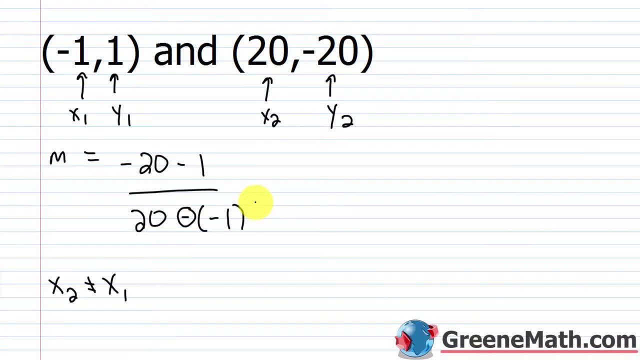 Mistake of just seeing that out in front and just putting minus 1.. You get the wrong answer. So then all I need to do now is just simplify. I have negative 20 minus 1,, which is negative 21. And this is over 20 minus a negative 1,, which is the same thing as 20 plus 1,, which is 21.. 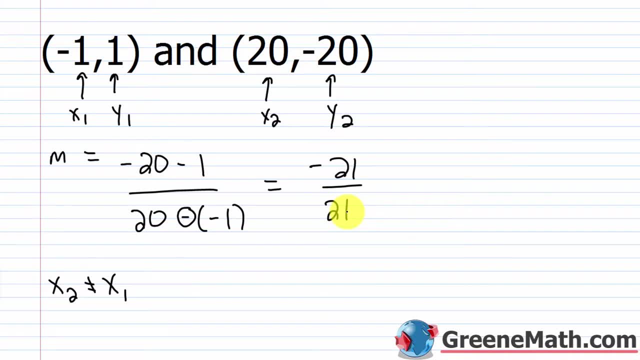 So I end up with negative 21 over 21,, which is the same thing as negative 1, right, Negative 1.. So m again my slope. let me label that real quick. My slope is equal to negative 1.. So let's see if we can make a little sense out of this slope thing. 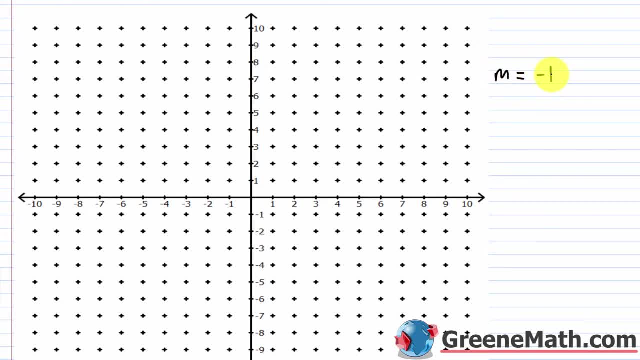 So we saw that m is equal to negative 1.. So what does that mean? Well, again, if you kind of look at the rise over run explanation- so rise over run- we know that we can write negative 1 as negative. 1 over 1, right, That's the same thing. If you divide by 1, it's just itself. So I can put this: 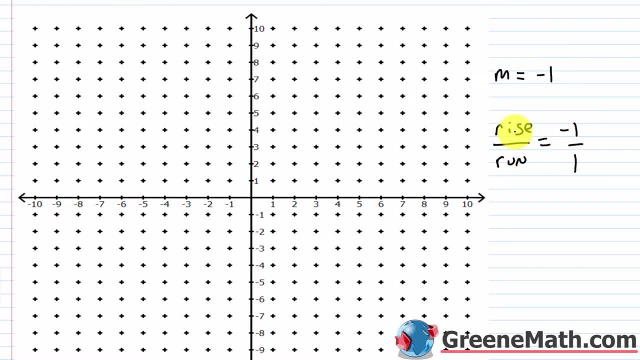 as equal to negative 1 over 1.. So I look at what's in the numerator: I have rise here and I have negative 1 here. So that means I'm going to rise by negative 1 or fall by 1 unit for every run which we think of as 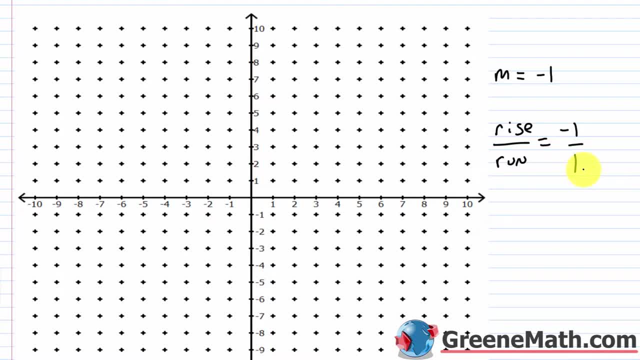 going sideways by 1 unit. Okay now, because this is positive down in the run, that means I'm going to the right. So positive in terms of the x-axis means you go right. Negative means you go left. Positives in terms of the y-axis. 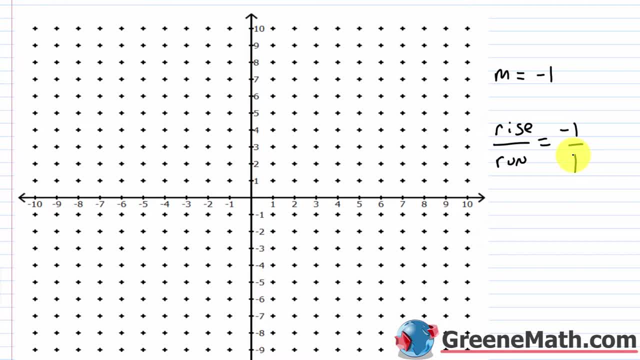 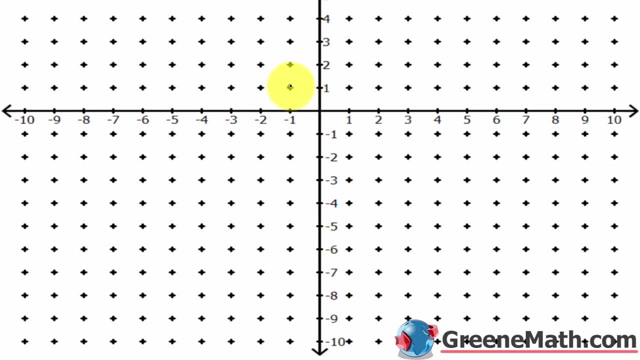 this means you go up, Negative means you go down. So if I started out at a point on this line, so we know that negative 1 comma 1, which is going to be right here, So that's a point on the line, I could actually use this to graph the line. 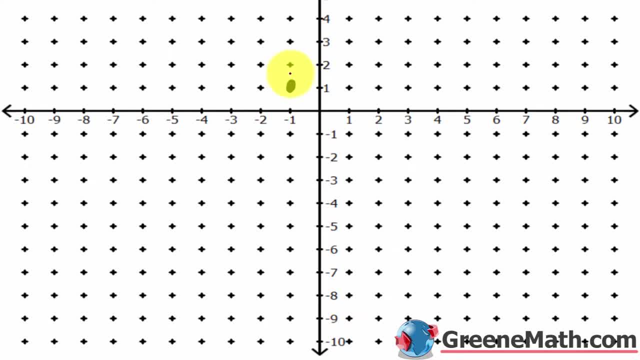 because I know that I'm going to fall by 1 unit, So I'm going to fall by 1 unit. thinking about the rise for every 1 unit, I go to the right, So I'm going to go down 1 and over to the right 1.. 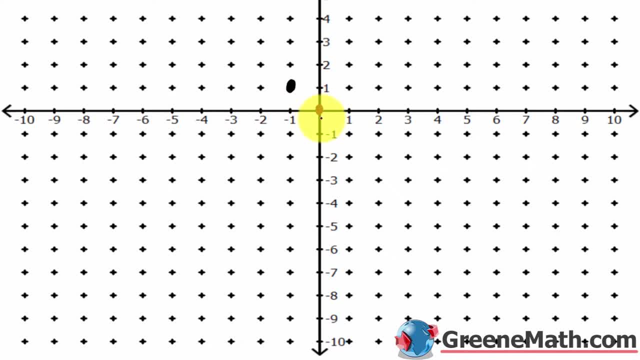 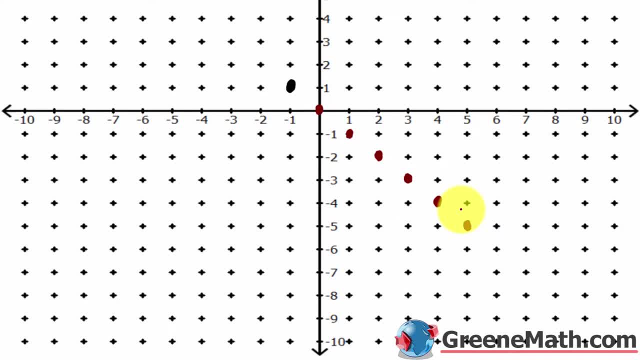 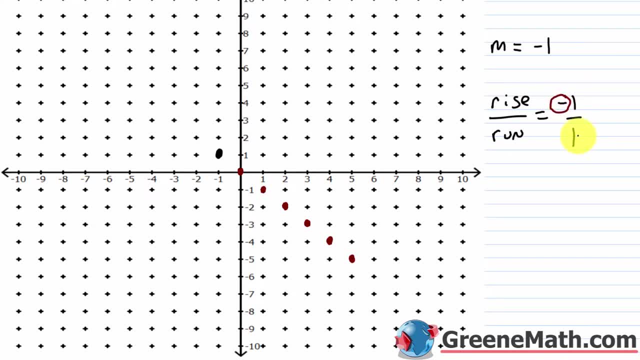 Or another thing I can do: remember, when we're dividing and we think about having a negative in the numerator but a positive in the denominator, I can legally switch that And I can legally say that this is 1 divided by negative. 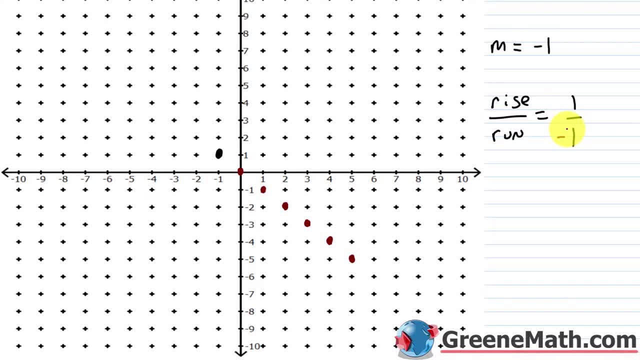 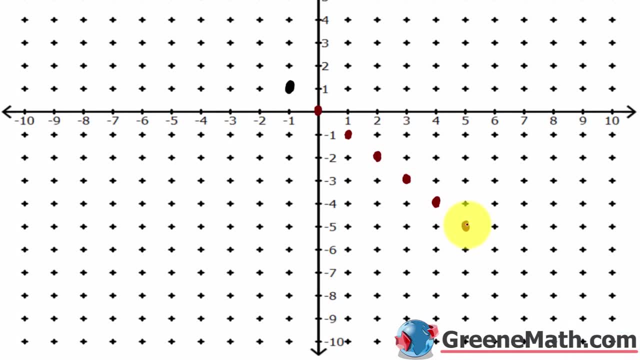 Now how would we read that? Well, that means that we would rise 1 unit for every unit we go to the left on the x-axis. So, starting out at this point, I would go to the left 1 unit and then I would rise. 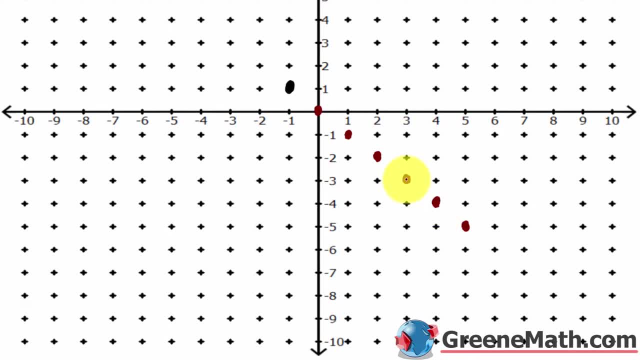 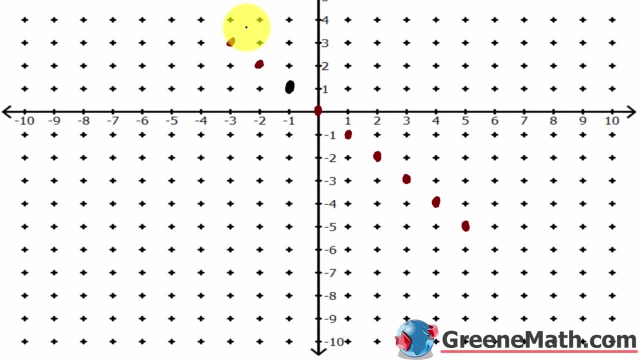 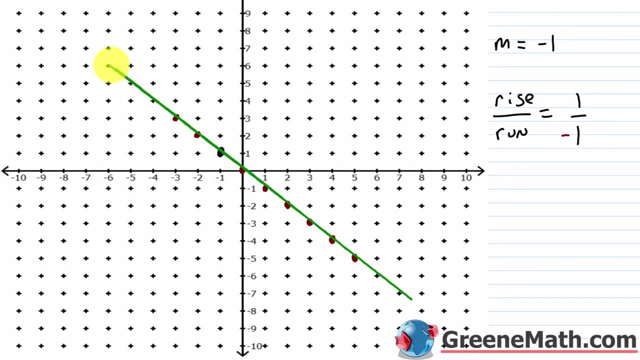 another point, And you can see that I can keep going, I can keep going, I can keep going. I can easily draw a completely straight line through those points. And let me do that real quick. Not perfectly straight, but you get the idea, And later on we're going to learn how to take this. 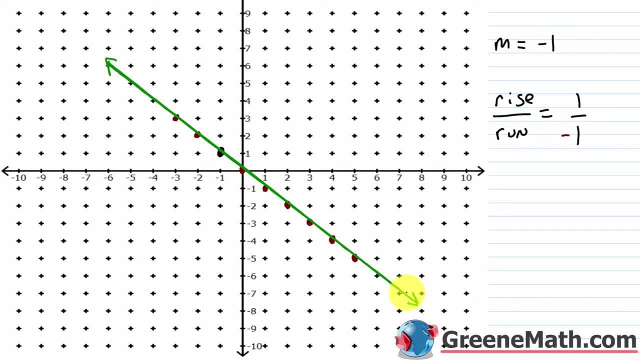 information that we have and find the equation for the line. So this is actually: y equals negative x, And I know this is going to be a lot of work, but it's going to be a lot of work, So I'm going to show that you don't know how to do that yet. That's okay, We're going to learn it very, very. 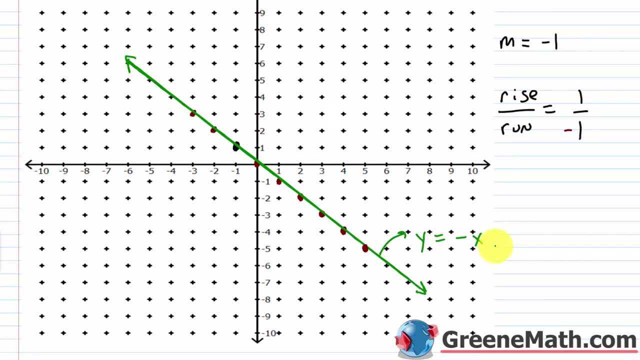 soon in the future. So quickly I want to show you that if I switched which ordered pair I labeled as x sub 1, y sub 1 with the ordered pair I labeled as x- sub 2, y sub 2, that it would make. 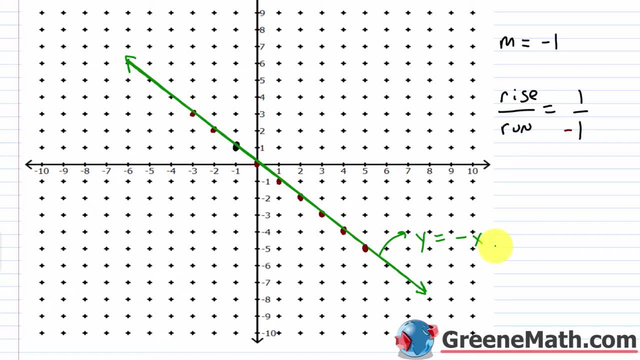 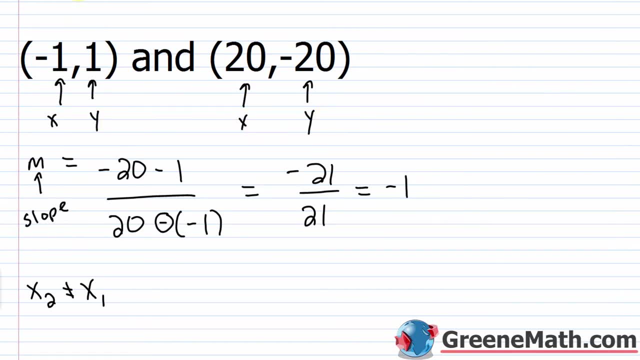 no difference and your slope would still be negative 1.. Let's do that real quick before we move on. All right, So let's just switch the way these are labeled, And so, instead of this being x sub 1, y sub 1,, it's going to be x sub 2, y sub 2.. 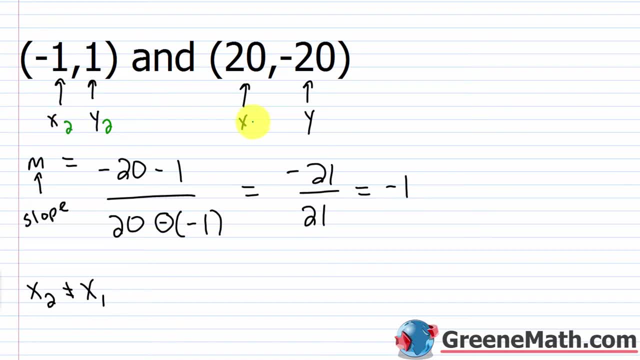 And this is going to be x sub 1, y sub 1.. And let me erase this real quick. So the slope formula again, it's m is equal to y sub 2 minus y sub 1 over x sub 2 minus x sub 1.. And let's just crank. 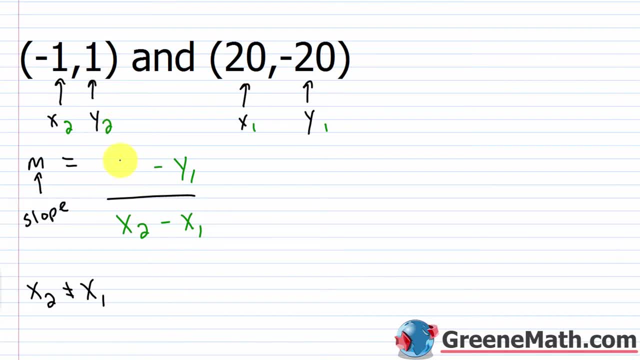 this out real quick. So y sub 2 is now 1.. So I'm going to plug that in. And minus y sub 1, y sub 1 is negative 20.. Again, pay close attention. You're plugging in a negative 20.. So that's going in. 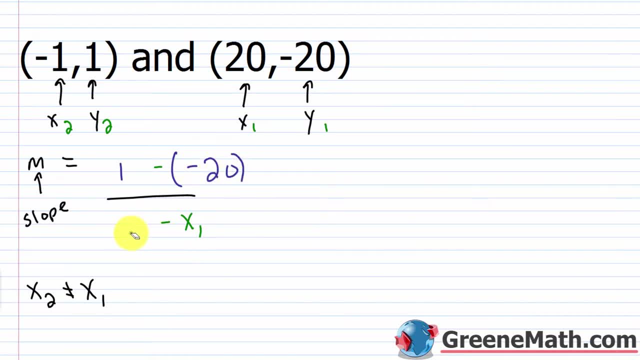 here, And then this is over x sub 2,, which is now negative 1, minus x sub 1,, which is 20.. Minus 20.. Okay, So what are we going to get? We have 1 minus a negative 20.. That's the same thing as 1 plus 20.. 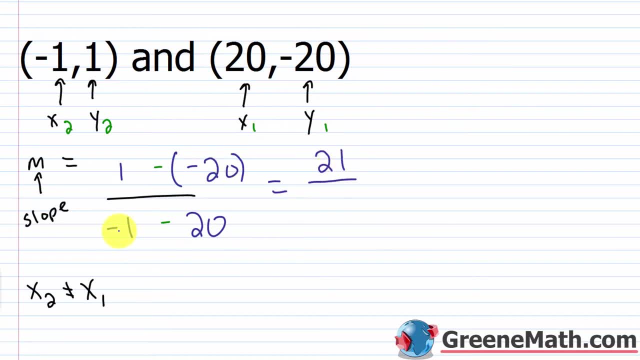 That's 21.. This is over. Here we have negative 1 minus 20, which is negative 21.. So again, you see, it's going to be the same thing: 21 divided by negative 20, 21 is negative 1.. So this is negative 1.. Or again, in terms of slope, we could think about: 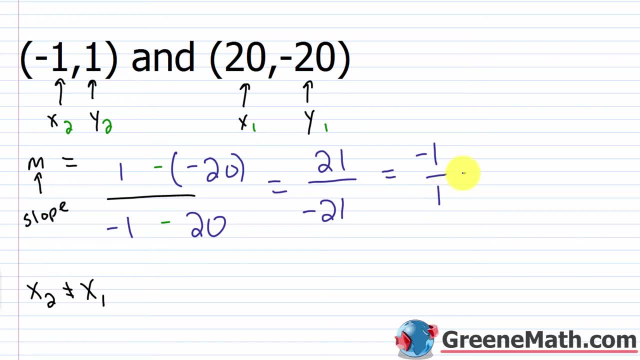 this as negative 1 over 1.. Or we could write it as 1 over negative 1, right Again, as it relates to rise over run. we've already seen that we can use that in two different ways. All right. 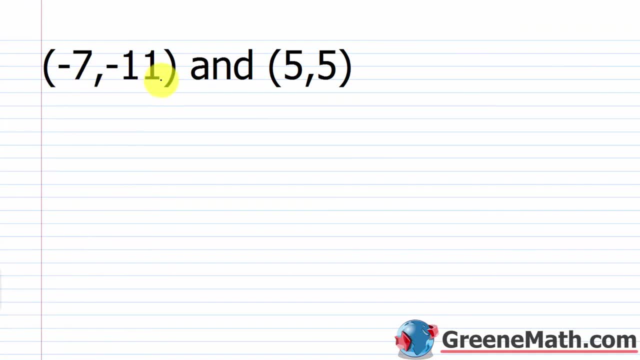 let's take a look at the next problem. So we have the ordered pair: negative 7 comma negative 11, and 5 comma 5.. So these two points are what we're given And we want to calculate the slope. So 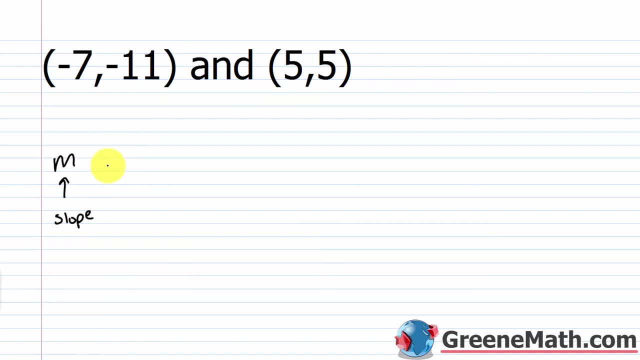 m. again our slope is equal to y sub 2 minus y sub 1 over x sub 2 minus x sub 1.. And again, x sub 2 cannot be equal to x sub 1.. So we're going to label our points And a general practice for me. 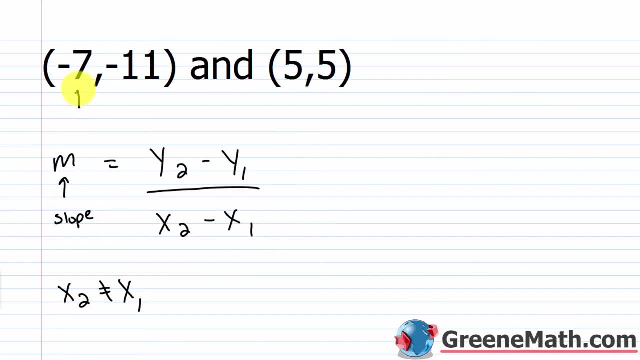 and probably for you, is just to label the first point as x sub 1, y sub 1.. And again, as I just showed you, it doesn't matter, You get the same answer either way And this one's going to be x sub 2. 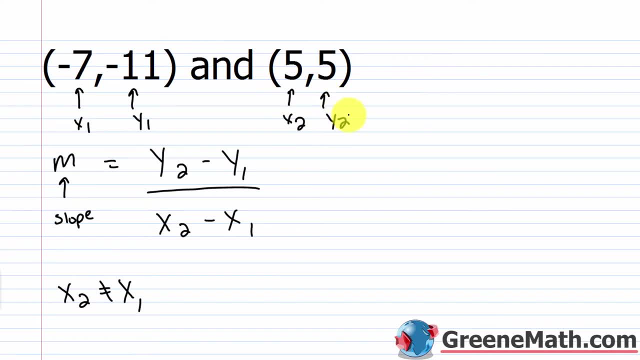 over y sub 2.. Okay, So y sub 2 is 5.. So let me erase that and put a 5. Minus y sub 1, that's negative 11.. Let me erase this and put negative 11.. This is over. We have x sub 2.. That's going. 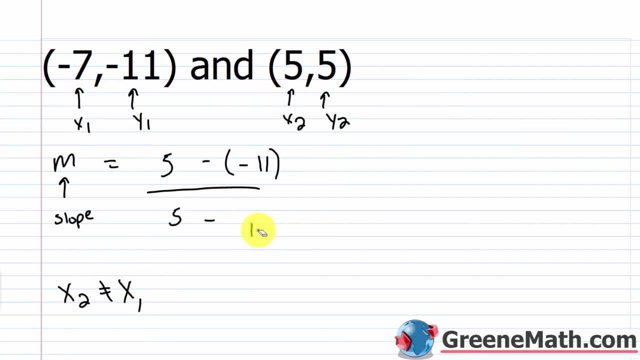 to be 5 minus x sub 1, which is negative 7.. So minus a negative 7.. So in each case here we have to pay close attention to our signs, because we have minus and negative. So 5 minus a negative 11.. 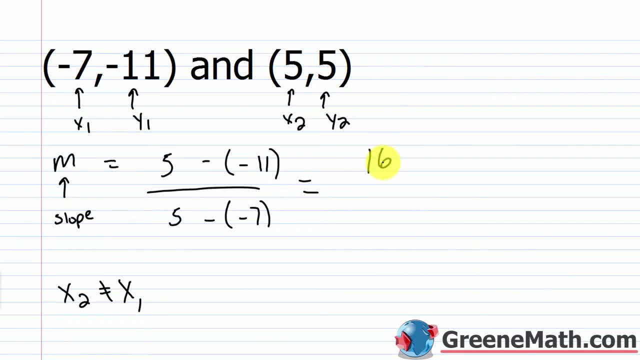 Is the same thing as 5 plus 11,, which is 16.. 5 minus a negative 7 is the same thing as 5 plus 7, and that's 12.. Now we can reduce this. Both are divisible by 4.. 16 divided by 4 is 4.. 12 divided: 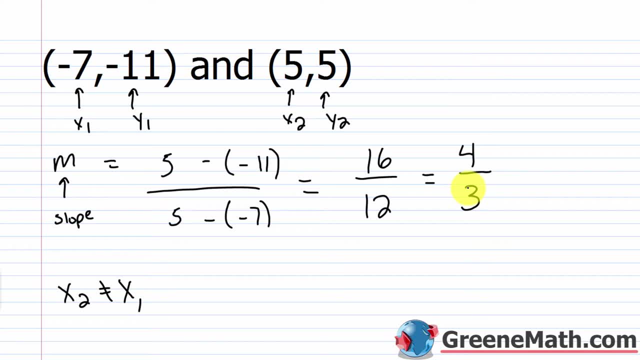 by 4 is 3.. So we get 4 thirds here, or 4 over 3.. Now we think about this in terms of, again, rise over run. So rise over run is equal to 4 over 3.. So that means that if I'm at a given point on a line, I can rise 4 units or go up 4 units. 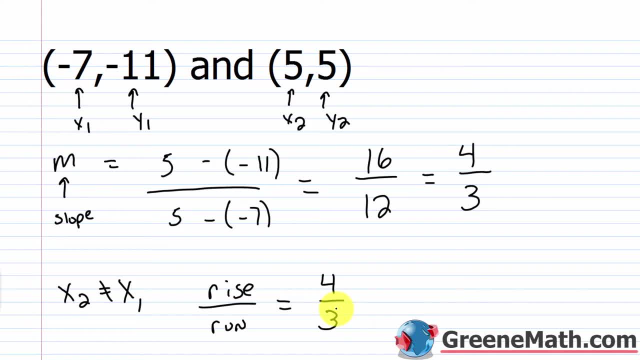 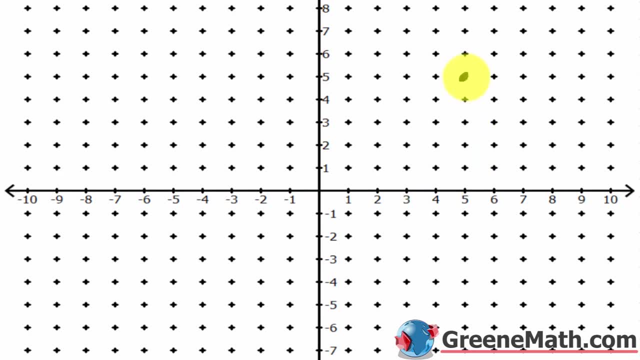 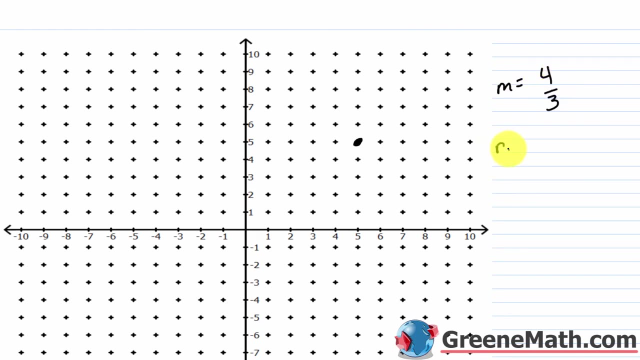 and then run 3.. So go to the right 3, and I'll end up at another point on that line. So a point on the line is 5 comma 5.. So that's going to be right here. Again, our slope m is equal to 4 thirds. So in terms of rise over run, this is 4 over 3.. 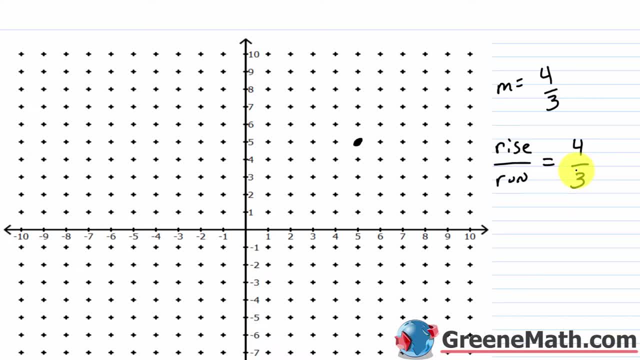 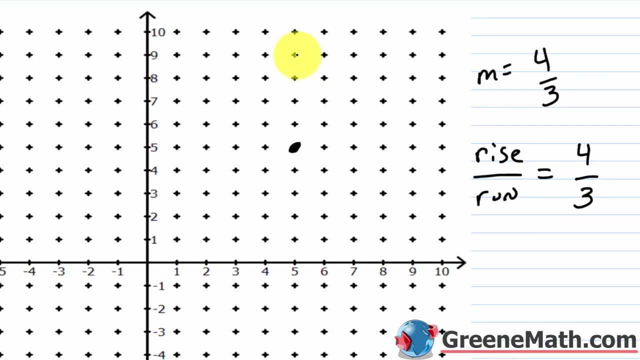 So if I wanted to find another point on this line, I could go up 4, so up 1,, 2,, 3,, 4, and then I could run 3.. Okay, when you talk about run again, positive means you go to the right, so I'm going to the right 3.. 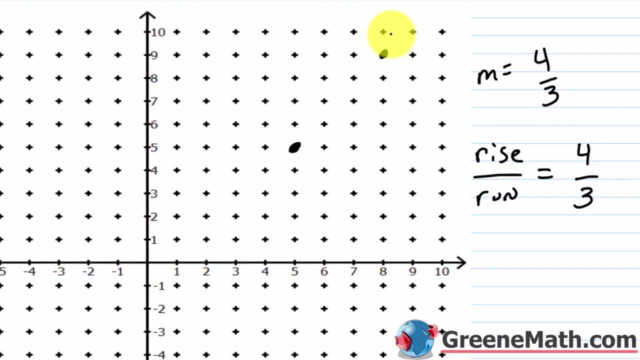 1,, 2,, 3.. So here's another point on that line. Now let's say you are out of space going up on your graph like I am. My kind of top number here is 10.. Well, no problem. 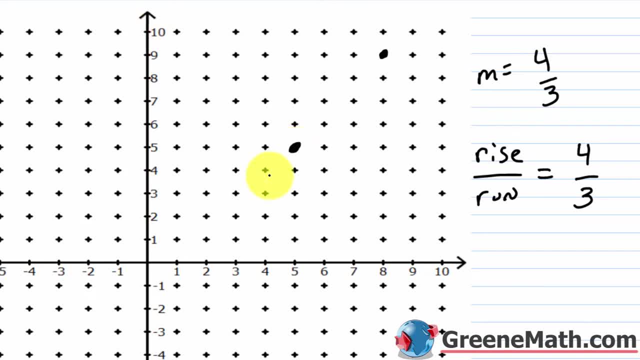 You could start at 5,, 5, and you can go in this direction. You might say: well, how do you do that? Well, one cool trick is to remember that a negative divided by a negative is a positive. So really I could write this as negative 4 over negative 3.. 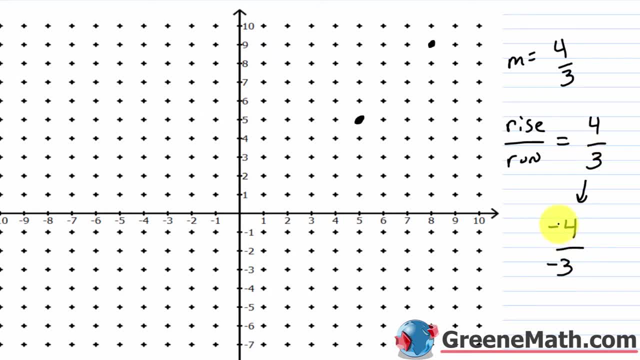 This has the same mathematical value as 4 thirds, because if I divide a negative by a negative, I get a positive, which is what I have here. So, using that thought process, I could start at this point and I could fall 4 units. right, That's what negative 4 means in terms of rise. 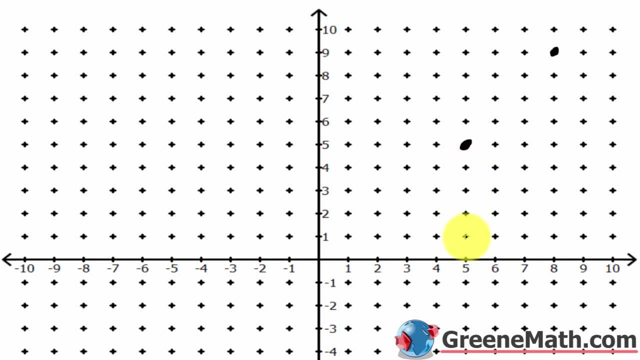 So I would go 1,, 2,, 3,, 4, and then I could go to the left 3 units. That's what negative 3 means in terms of run right. I'm going to the left, So 1,, 2, and then 3.. 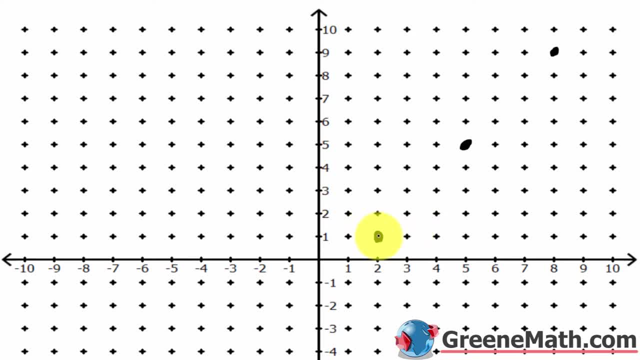 So here's another point on the line, and I could do that again. I'm going to fall: 4. 1,, 2,, 3, 4.. I'm going to run to the left: 3. 1,, 2, 3.. 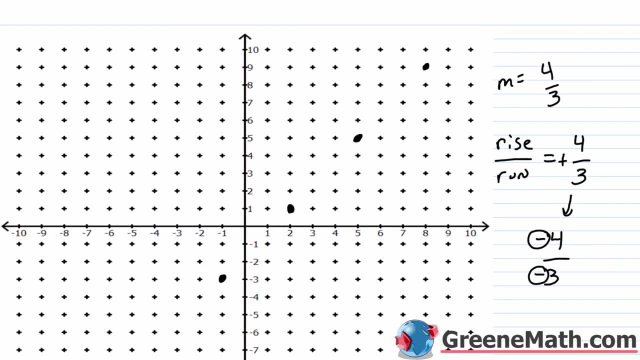 So here's that, and then I could graph this line if I wanted to. Okay, and again, not perfect, but kind of the best I can do, All right. and then what's the equation for this line? Again, I know that you don't know how to figure that out yet, but I'm just going to go ahead and give it to you. 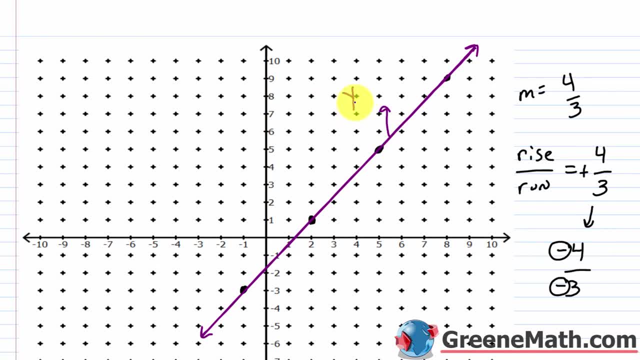 And so this would be the graph, for y equals 4 thirds, x minus 5 thirds, And again, really shortly, we're going to learn how to do that. All right, so, as you may or may not have figured out at this point, 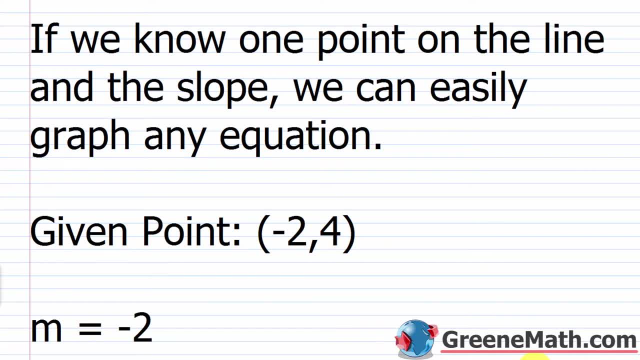 if you know one point on the line and the slope, we can easily graph any equation And this is kind of the preferred method to do it. You saw kind of in the last lesson we were going to go through and make these ordered pairs. 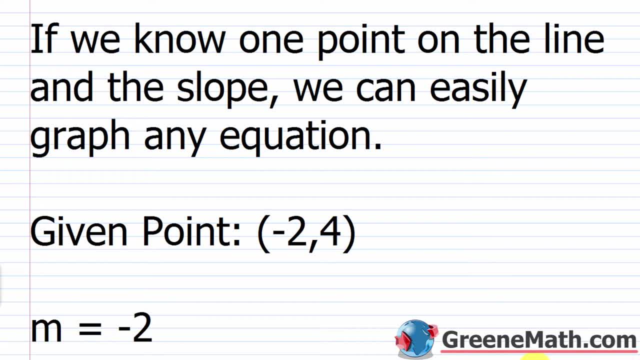 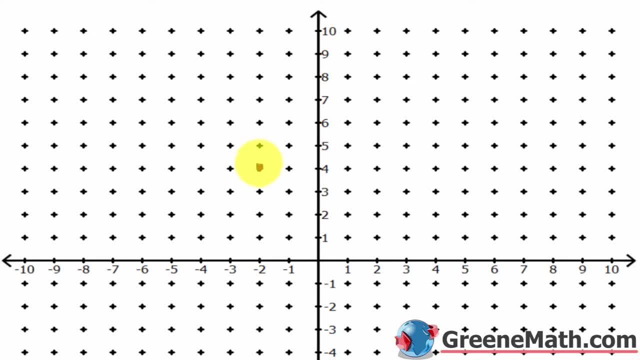 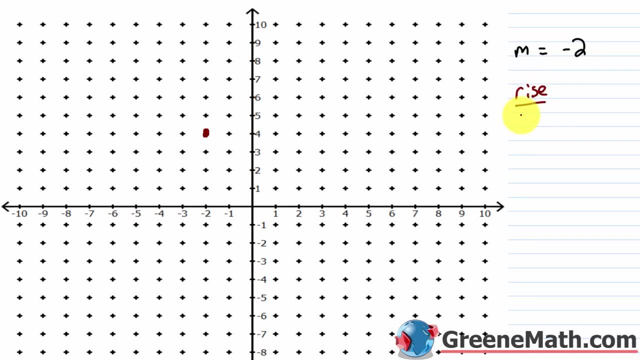 So here's negative 2,, here's 4, so that would be negative 2 comma 4.. And if my slope is negative 2,, again, that means that my rise over run is equal to negative 2 over 1.. 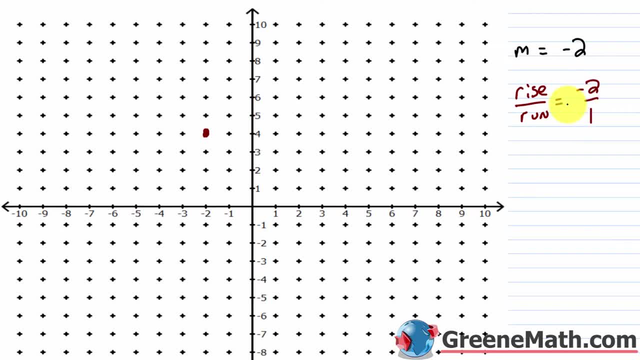 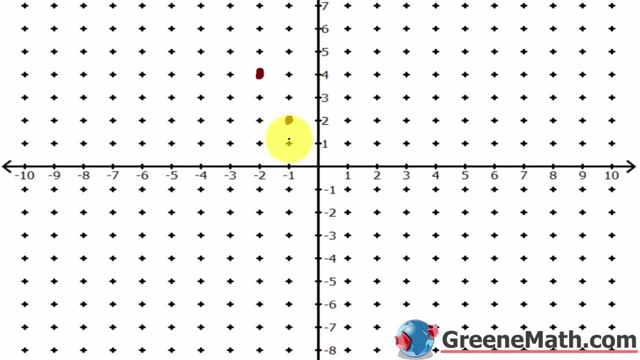 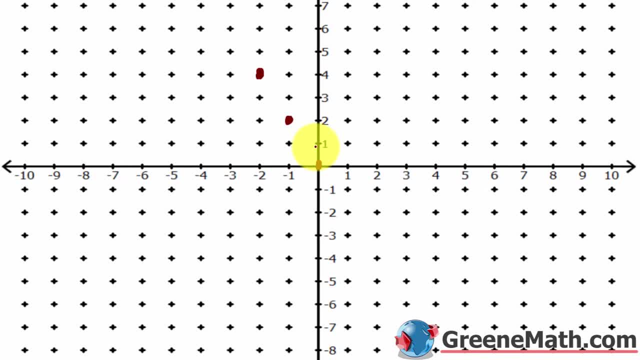 And once you have that you're going to be able to do this. But once you have 3 points- really 2, you can draw the line, But 3, again is nice to get a nice clean line, And I like to do a few more actually if I'm freehand. 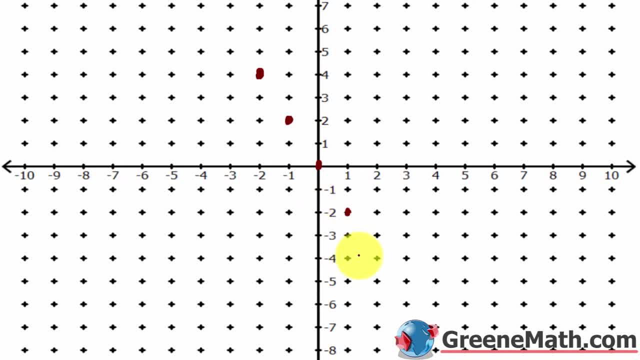 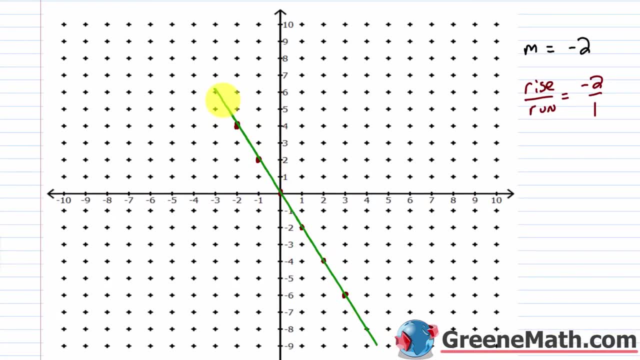 So 1, 2 down, 1 over 1, 2 down, 1 over to the right, 1, 2 down, 1 over to the right. So kind of a faster way to graph a line. 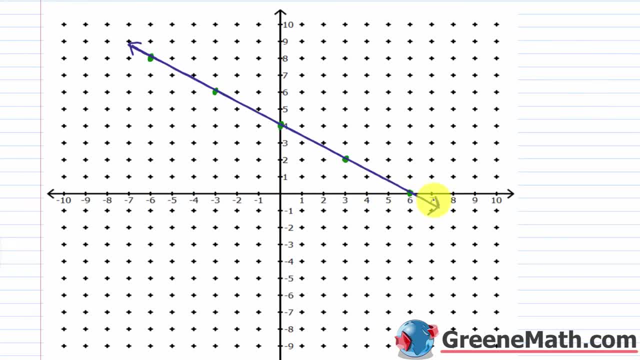 OK, so another thing we want to talk about. OK, so another thing we want to talk about. let's say, you get to your homework and you're presented with a graph and so the graph of this line. they have some clearly indicated points and it asks for the slope of the line. well, using the 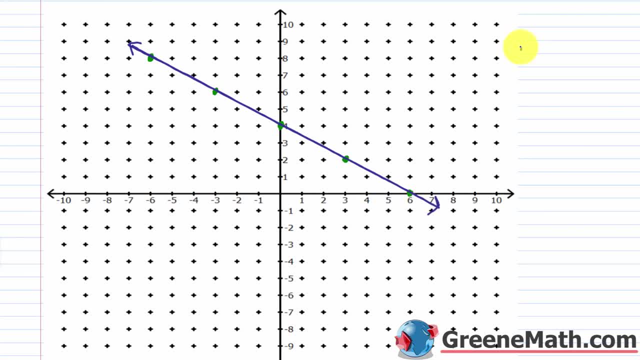 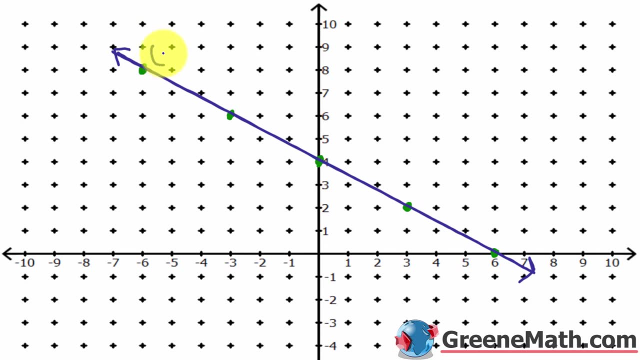 rise over run kind of thought process. so rise over run, you can calculate it. so let's say you start at one of the points. so this point right here looks like negative six comma eight. so negative six comma eight, all right. so you think, what would i need to do to get to the next point? so how much? 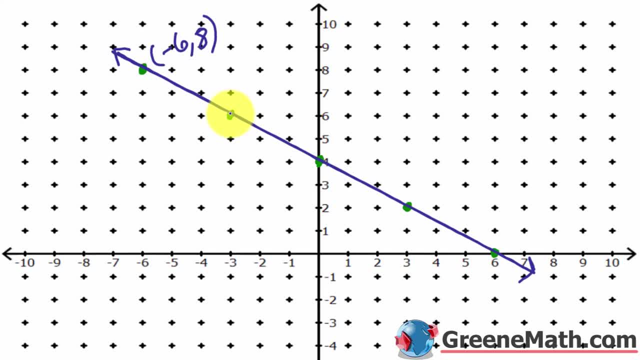 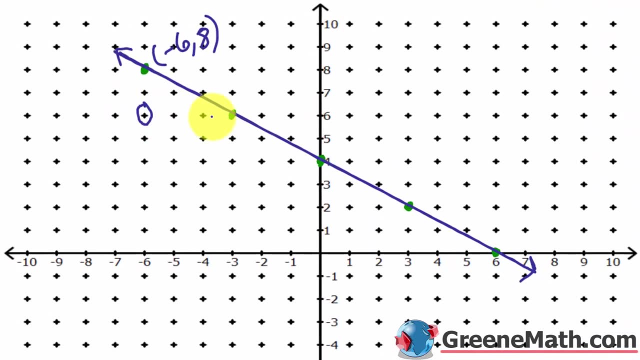 do i rise? so to get over here, i've got a fall right, so i'm rising by a negative amount. i'm going down one, two units. so right, here is not the next point, but it's the same y location as the next point. so that means I'm falling by two units and then I'm running over to the right, which is 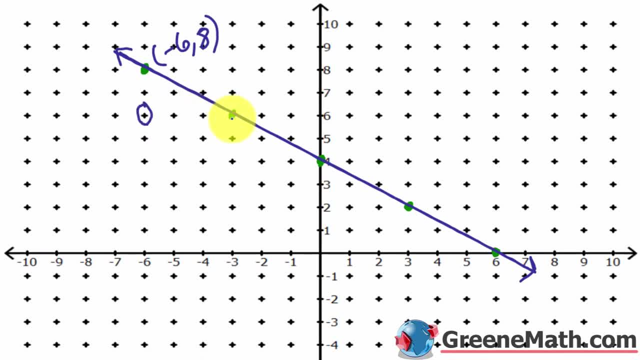 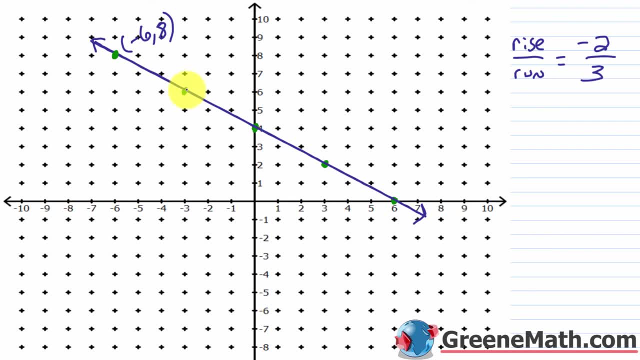 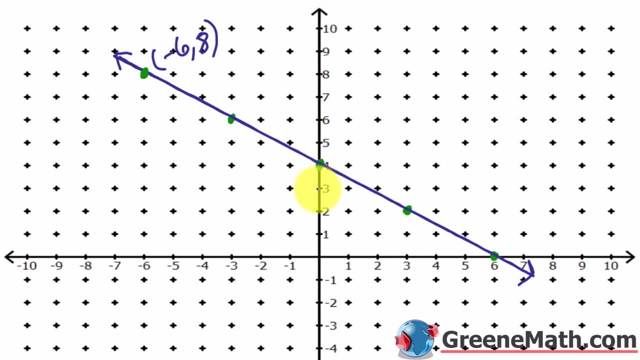 positive. I'm going over one, two, three units to the right. so my slope is negative, two-thirds, and then you can check that again, starting at the next point down to one, two go over to the right, three. one, two, three. and I'm at the next point down to one, two over to the right, three, one, two, three. I'm at the. 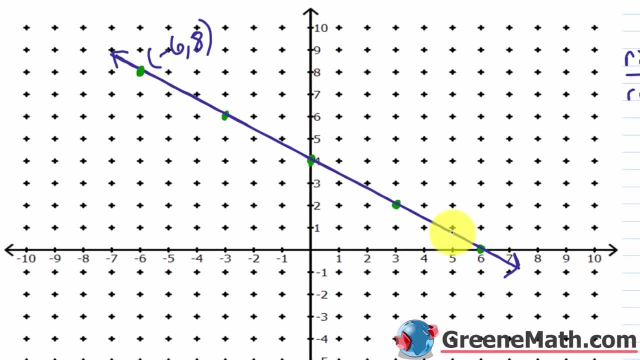 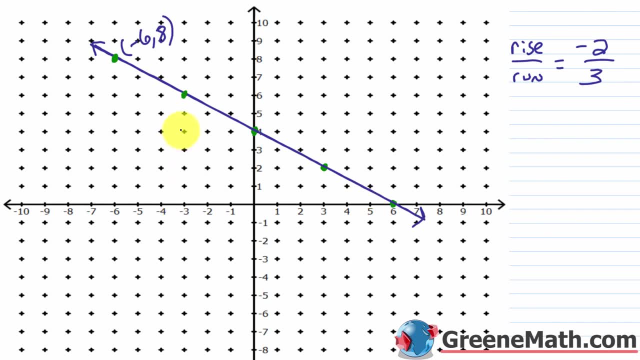 next point. again, you can keep doing that. so our slope in this case is negative two-thirds. and then one of the other ways you could check this, you could look at one of the other points. so this point right here is negative three comma six. so negative three comma six, and you could use your slope formula and 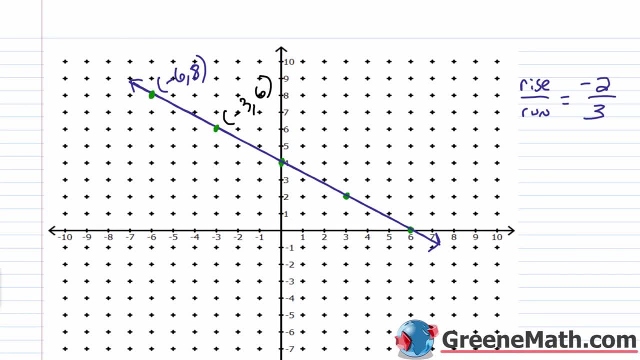 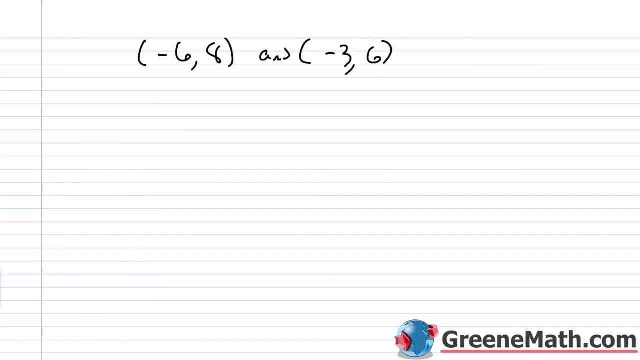 see if you get a slope of negative two-thirds. let's do that real quick. so remember your slope. formula M is the slope. this is equal to Y sub 2 minus Y sub 1, over X sub 2 minus X sub 1. again where X sub 2 does not equal X sub 1, and I'm just going to go ahead and 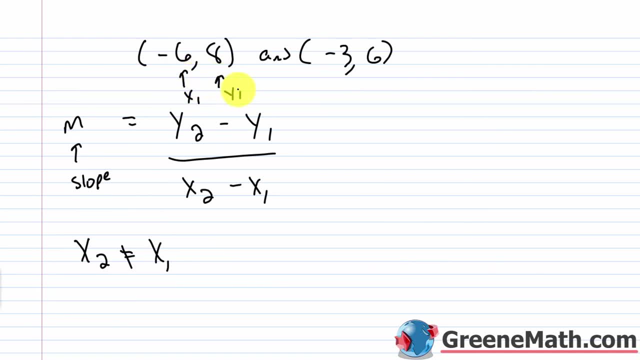 label this first point as X sub 1, Y sub 1, and the second one as X sub 2, Y sub 2, and again, if you wanted to change that around, you get the same answer. so Y sub 2 is 6. so I'm going to erase this and put a 6: Y sub 1 is 8. 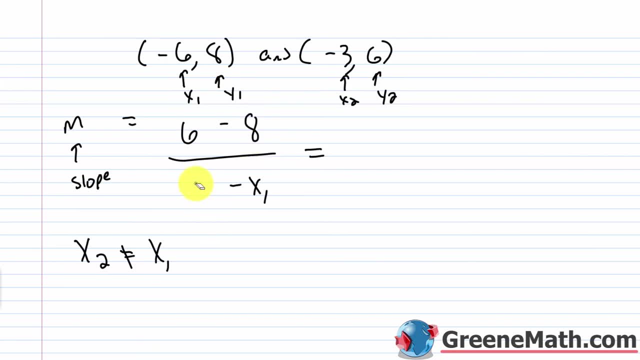 I'm going to erase this and put an 8. X sub 2 is negative 3, so I'll erase this and put negative 3. and X sub 1 is negative 6, so I'm going to erase this and put minus negative 6. or you can just do this right now and just say this is plus 6, so 6. 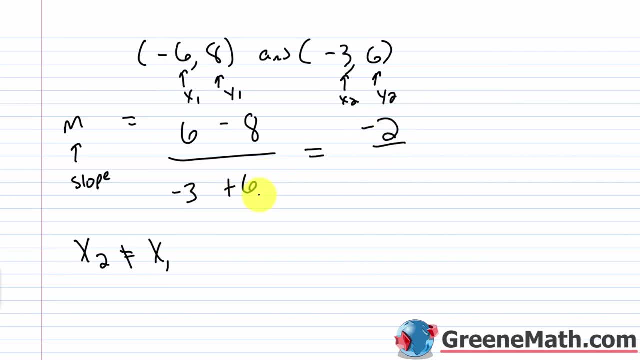 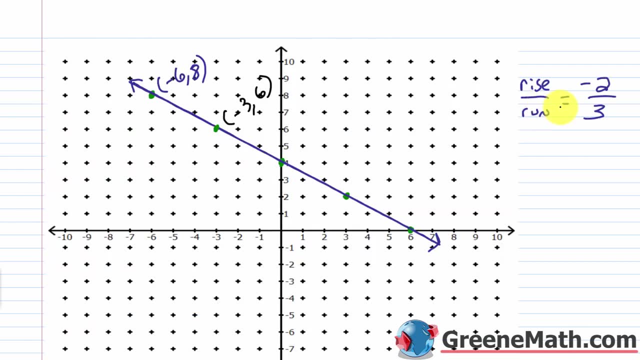 minus 8 is negative 2 and negative 3 plus 6 is 3, so you get negative 2 thirds as your slope and again that's exactly what you calculated here. your rise over run is equal to negative 2 thirds, or negative 2 over 3, all right, so 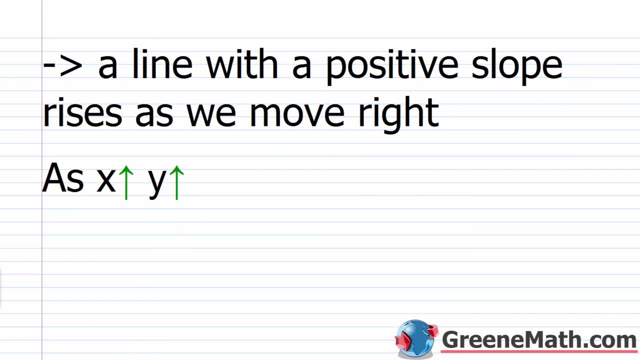 now that we have the base, we're going to do is we're going to do is we're going to start with the slope, and we're going to start with the slope. so let me just go ahead and put our basics down. let's wrap up our lesson with a few basic. 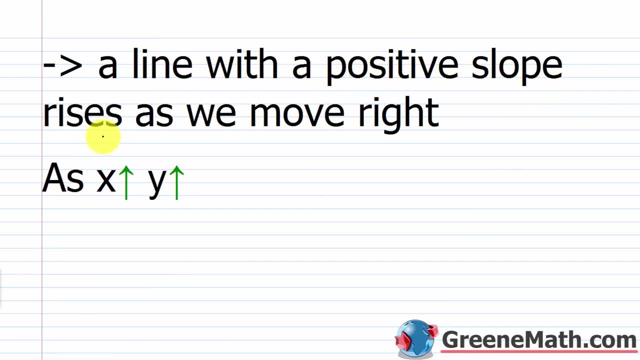 things that you need to know about slope. so the first thing is that a line with a positive slope rises as we move to the right, so that kind of looks like a line that does this right. so as we move to the right, so as X increases- remember, X increases going to the right- y increases, so as we go to the right, the 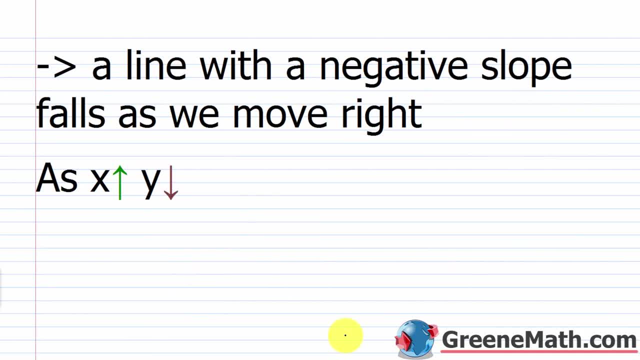 line is increasing in value slope falls as we move to the right. So in this case, as x increases, y is now going to decrease. So that line would look something like this: So as x is increasing- remember x increases as we move to the right- y is now decreasing. Your vertical values are moving down as we go to the. 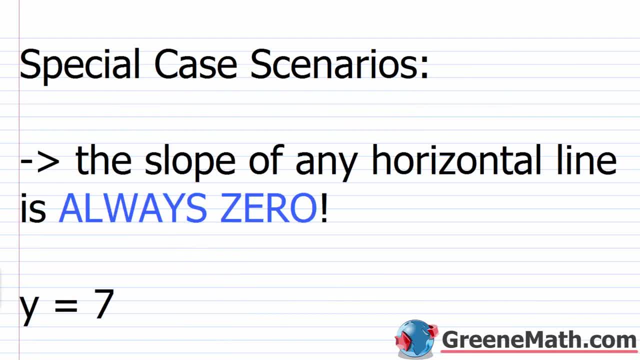 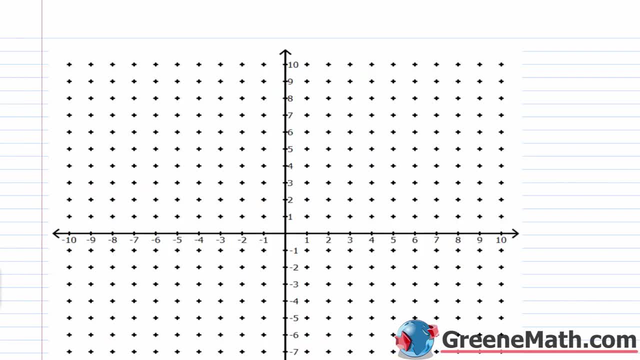 right. All right, let's talk about some special case scenarios. The slope of any horizontal line is always zero. So you have something like y equals 7.. So you'll recall graphically, I just find 7 on the y-axis and I draw a horizontal line. That's how I graph that. Okay, so this: